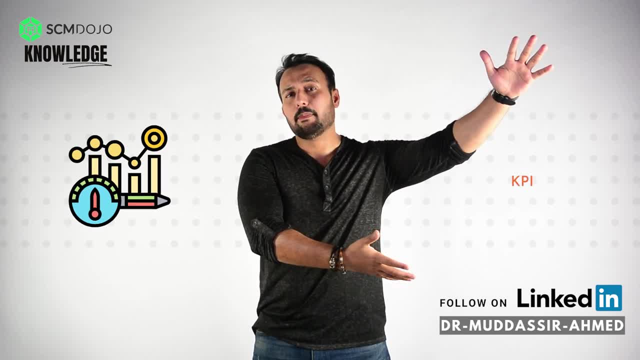 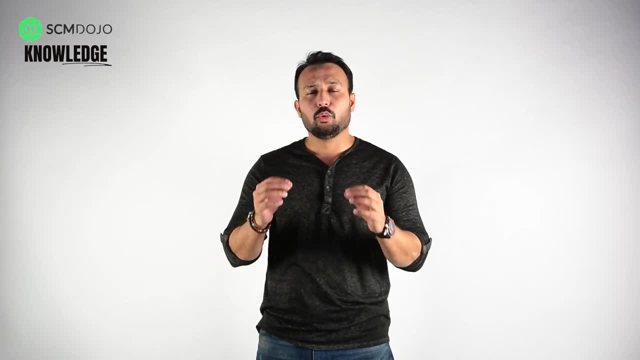 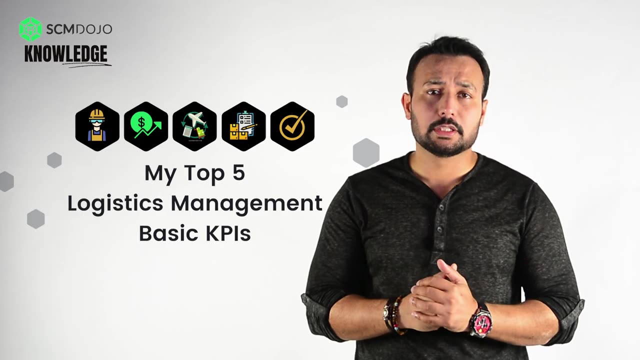 managers or the team leaders, creating a big list of KPIs like 18,, 19, and some of them don't even use any. So what I'm going to do is, today, I'm going to explain you top 5 basic logistics management KPIs which you should deploy, and that should cover most of the important things. 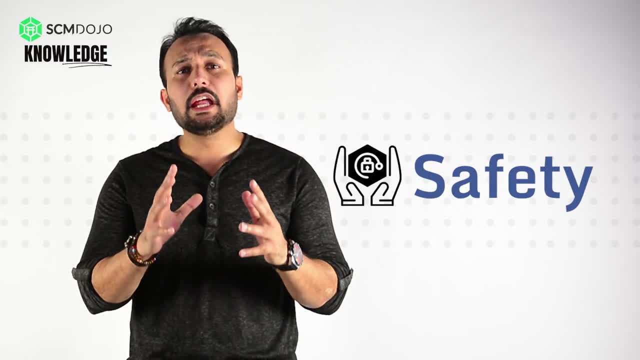 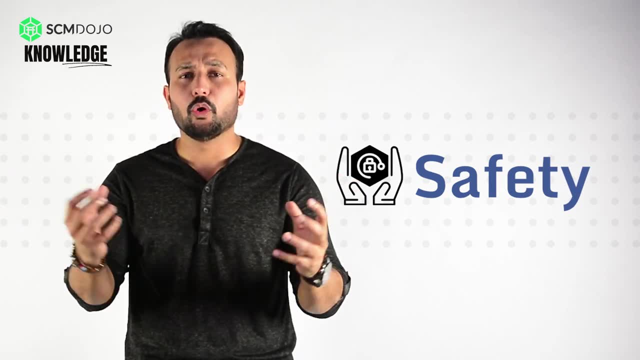 So let's begin. The first one is safety, And it is very important, right? What do you want as a supply chain? What do you want as a supply chain? What do you want as a supply chain Managers, logistics managers or a logistics team leader, that the employee coming into your 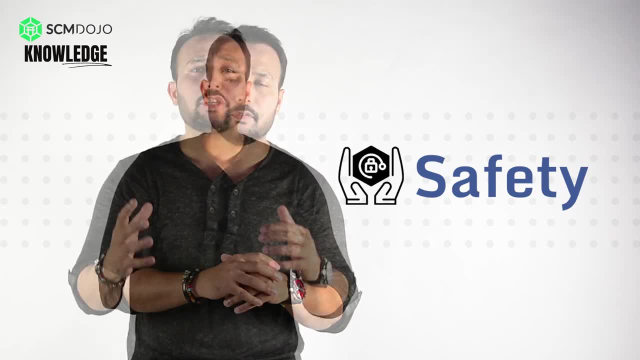 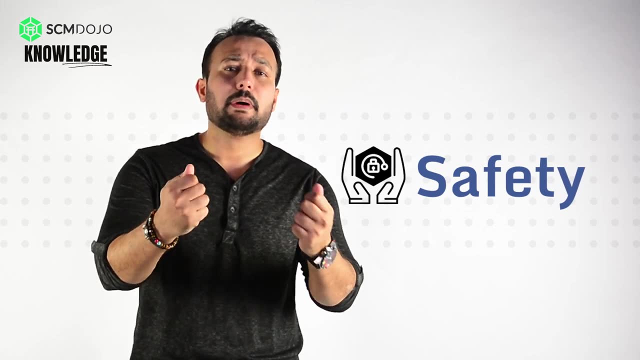 warehouse and your logistics environment. they are safe. As a team leaders and a manager is our responsibility to provide the most safe working environment, And we have to lead by example. What does that mean? That means we have to wear the PPEs, the highways, the helmet, the shoes, 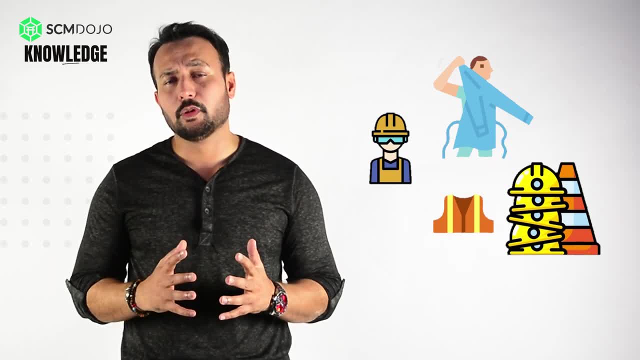 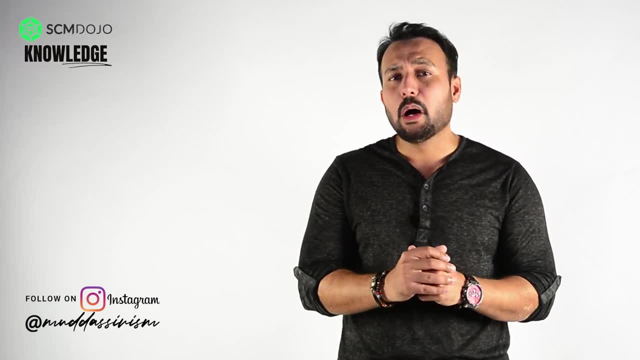 the whole lot. If we lead by example, then everybody else will follow. What is the safety KPIs? There are quite a few. which is a zero incident, A days away case rate or a near miss? I would say you can use any of them or one of them. It's. 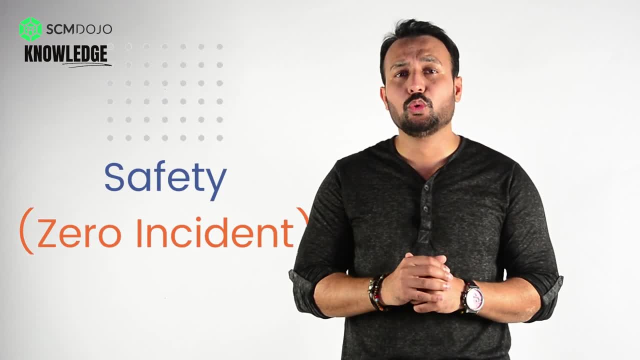 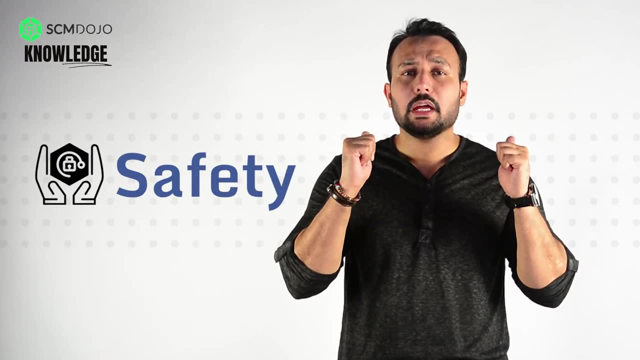 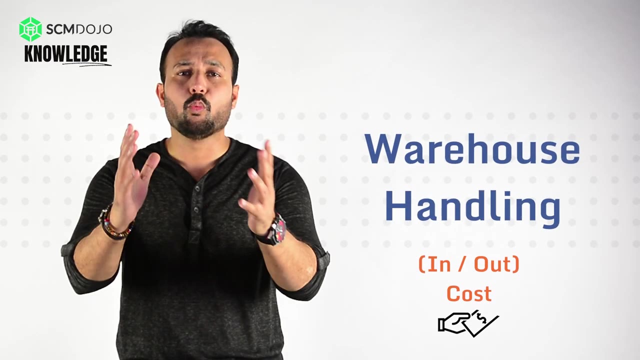 equally fine. What I generally recommend to do is to use the zero incident right, Which is zero incident, since how many days would be a good KPI to follow? So safety is the top most priority. Please keep it that way. The second one is the warehouse handling in and out cost. What does 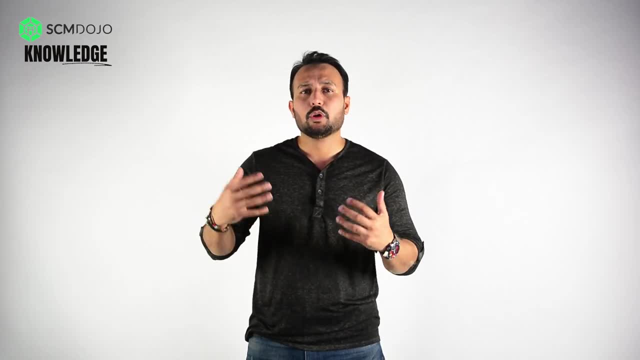 that mean. So when the shipment arrive at your warehouse, so your people go in and they basically de-stuff the container. So when the shipment arrive at your warehouse, so your people go in and they de-stuff the container or the truck and they basically put into the shelves. So that is. 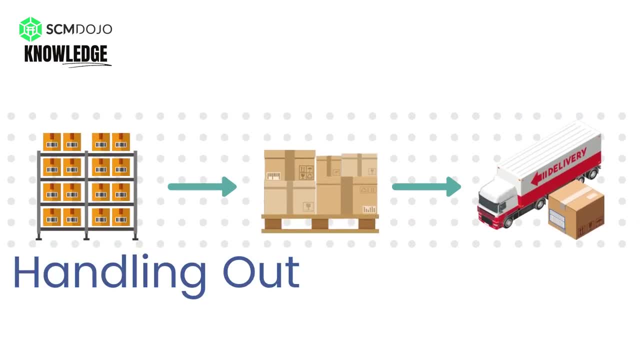 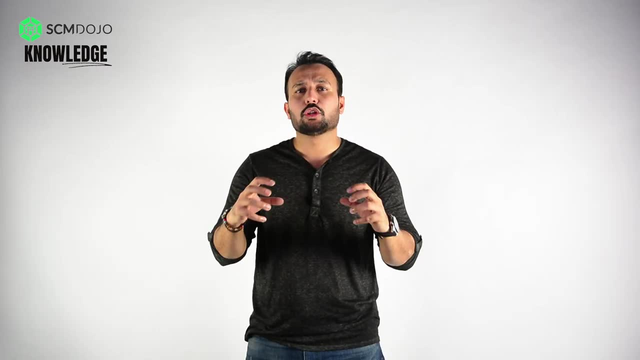 handling in right When the shipping out is. basically they're picking the product, they're packaging it and then they're putting back into a truck or a container. So this is handling in and out. So this is the cost where you should be estimated that how many labor hours is. 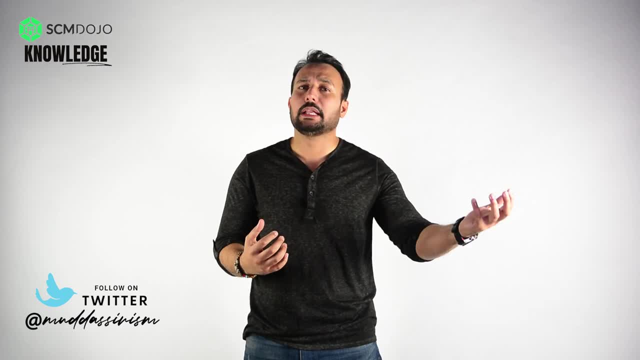 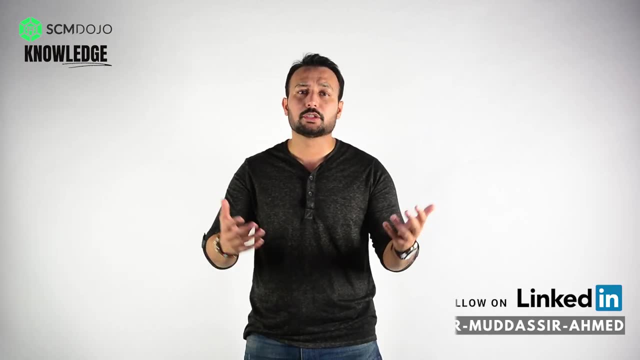 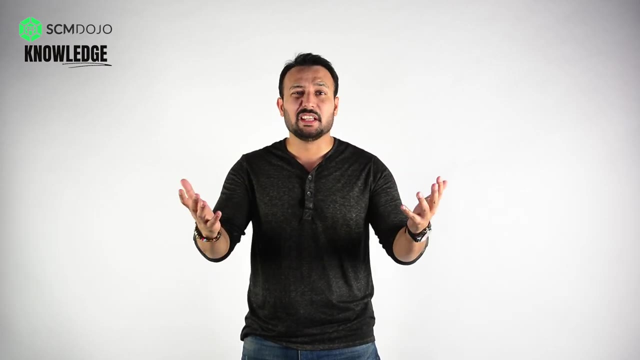 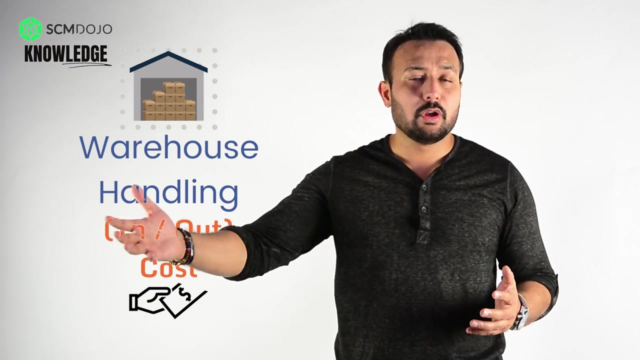 going in for product to handle in or handle out, And that would also important when you are negotiating your contract with the 3PL, because some of the 3PLs charge more than others. So if you have your own warehouse, maybe this is one of the important criteria If you're trying to. 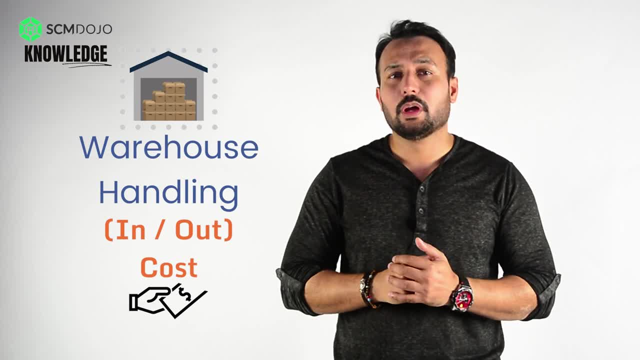 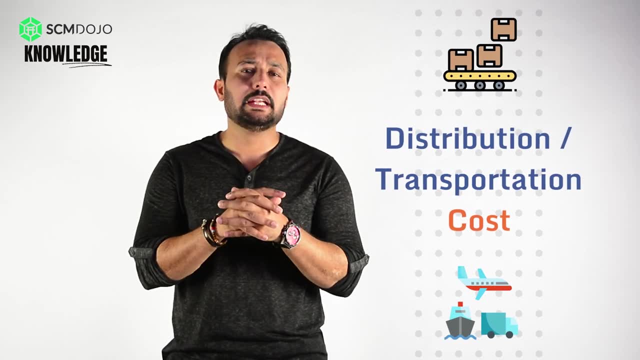 outsource it to the 3PL or somewhere else. So make sure you have this KPI available Number. third is distribution and transportation cost. Again, that cost is heavily dependent on the freight mode: If you're air freighting, if you're sea freighting. So this is very important. 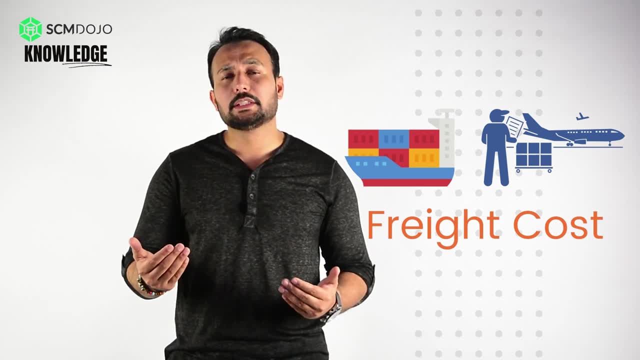 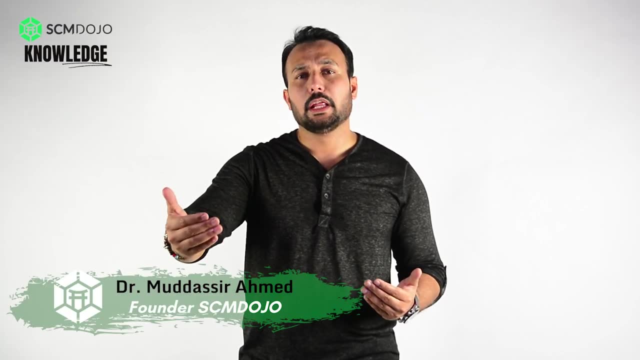 to understand. So, if you're air freighting, if you're sea freighting, if you're air freighting, so in a typical fashion, I would like to understand in this KPI that what is the cost of the container I have paid from China, Thailand, Japan, wherever? what is the terminal handling? 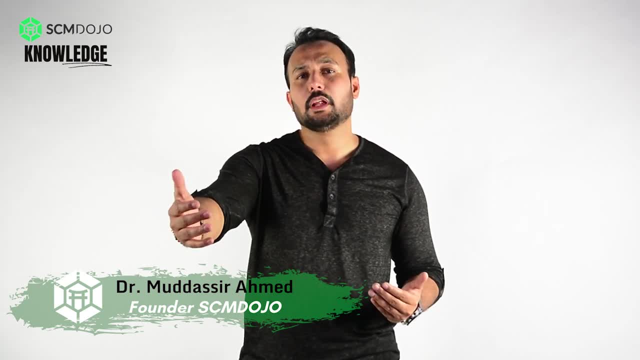 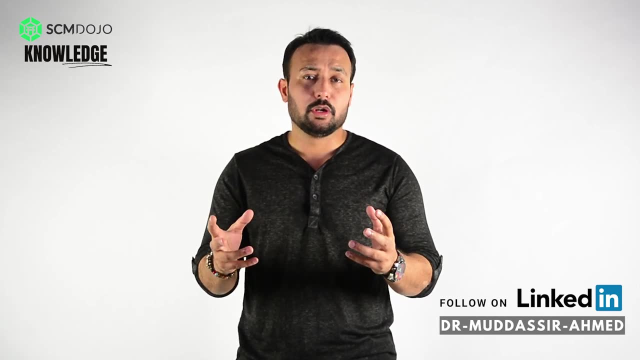 charges. then what are the charges I have paid for the truck from the terminal to arrive it at my warehouse? So this is my total transportation cost, which I like to understand. Number four is inventory accuracy. It is very important because if you're losing inventory and 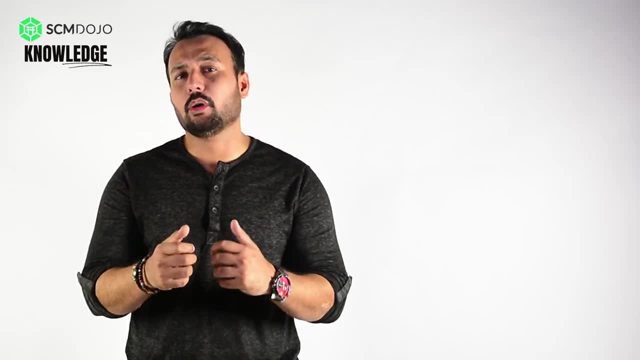 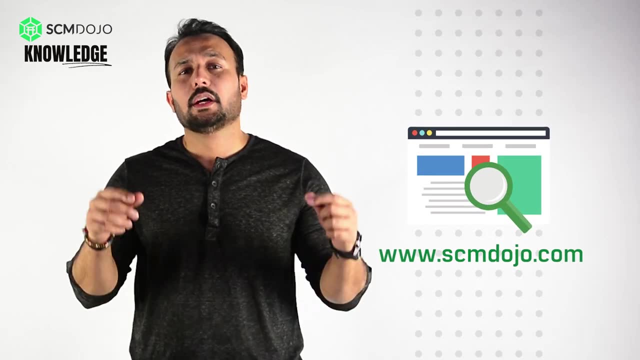 you can't find it when you want to pick it is a problem. So either you use a cycle counting or you do your annual stock take In SM Dujo. I've written a guide on that So there's a link below, or you can go to SM Dujo, click on guides and you will. 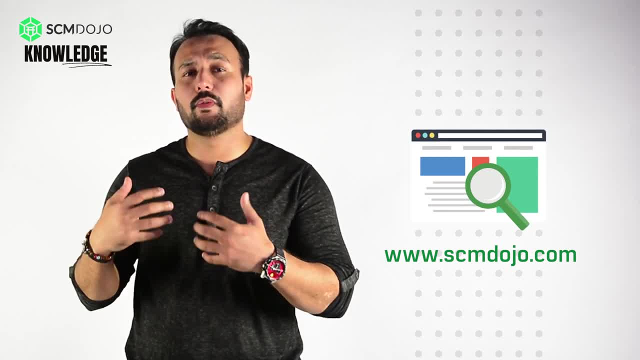 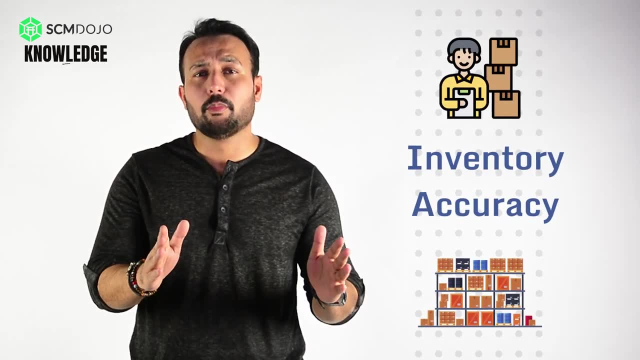 find a very interesting guide of a cycle counting and you will find the best practice of the stock taking. So you can get both of them, and I've provided the link below as well. So inventory accuracy is super important. So if you start losing inventory, that means there is a high 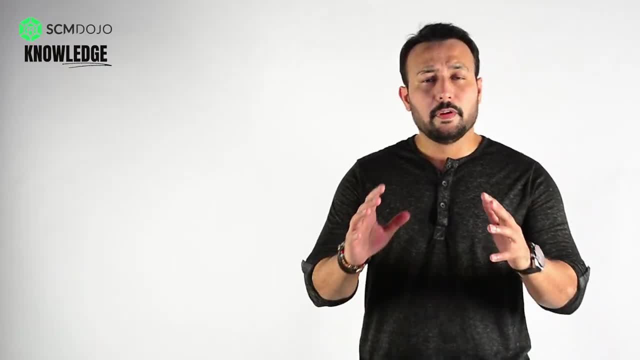 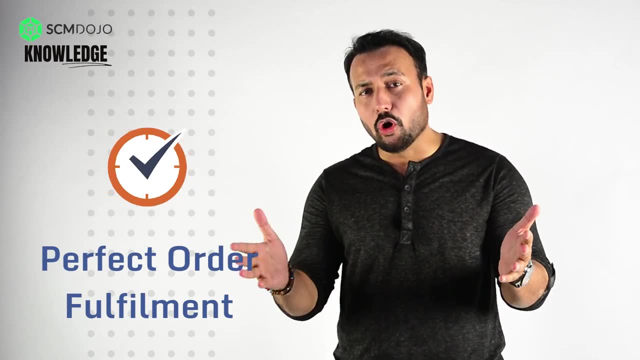 chance you cannot provide a good customer service. Number fifth, which is a slightly complicated, which is perfect order fulfillment. What does that mean? That you have delivered complete, you have delivered on time and you have provided all the right documents, right. So it's as I said, it's slightly. 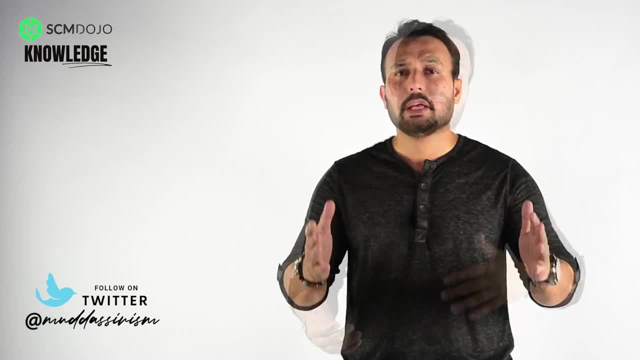 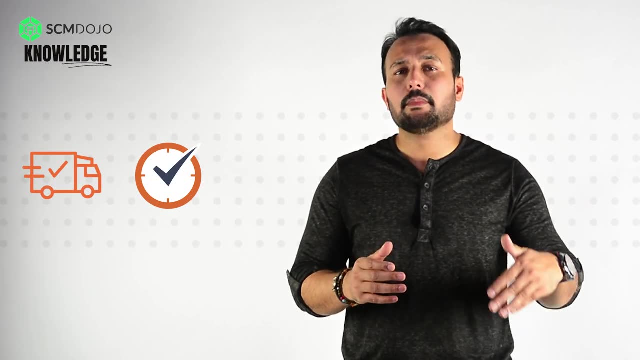 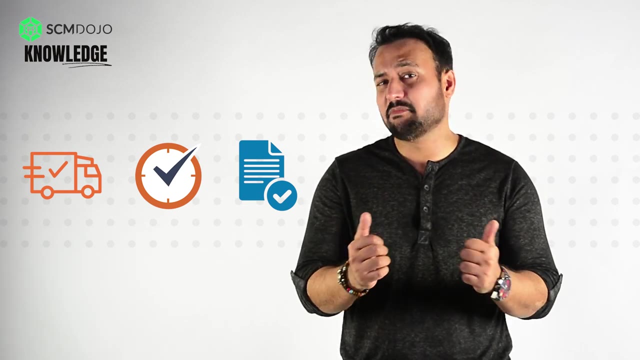 complicated. So what you do, what, how you measure is, for example, if a customer has ordered, you know, a hundred pieces of fans, or if you make fans, then you have delivered on time, in full, and provided all the required documentation for them to accept in the warehouse, And that is literally. 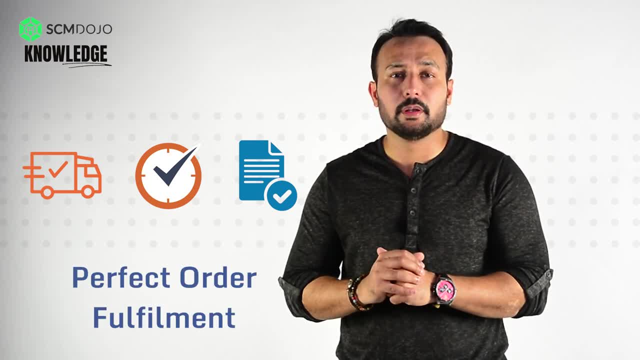 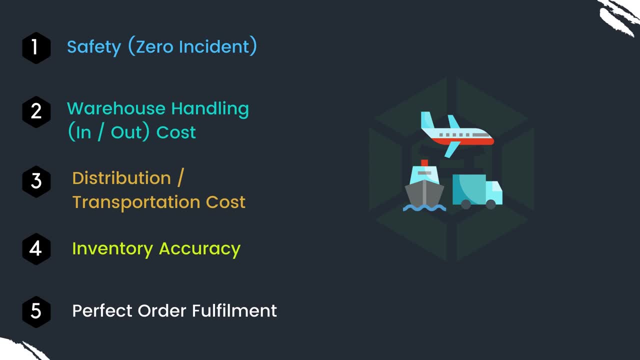 as simple as that. You can calculate your perfect order fulfillment. So hopefully you like the five KPIs I mentioned, which is a safety, a handling end cost, a transportation cost, inventory accuracy and, lastly, perfect order fulfillment. So if you want me to make more videos of this kind,